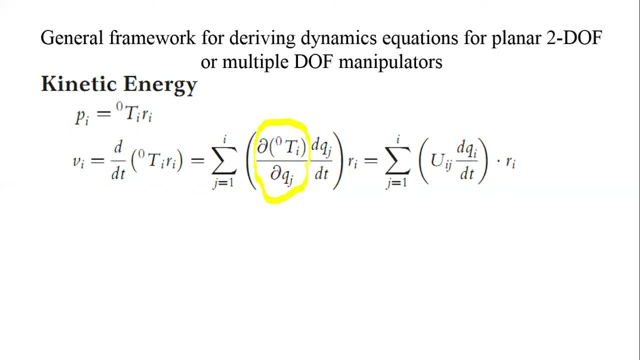 is going to be constant. This term del 0 ti by del q j is denoted by another term, u i j Voices. what are available to us now For the i-th link? the velocity of its link will have three components: x, i. 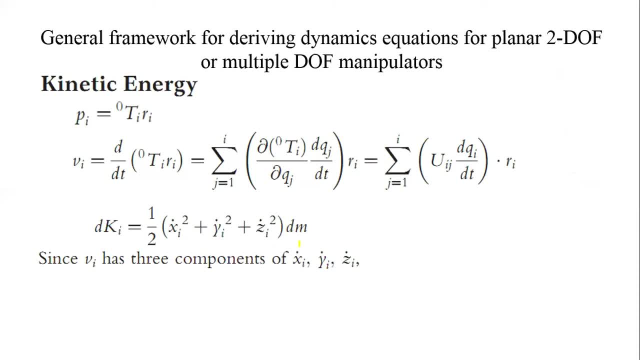 dot, y i. v i has three components that are x i dot, y dot and z i dot. the multiplication of v i with v i transpose will be equal to a matrix of three by three sides. now if we take the trace of this matrix then we can denote this expression or we can substitute this expression. 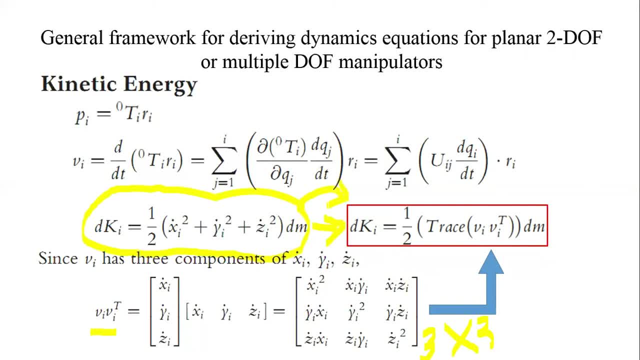 in this form. so d k i will be equal to half trace of this matrix. that means x? i dot square, plus y i dot square, plus z i dot square, which is basically equal to this thing into d? m. we know the expression of v? i in terms of d? q i by d? t? u, i, j and r? i. if we substitute: 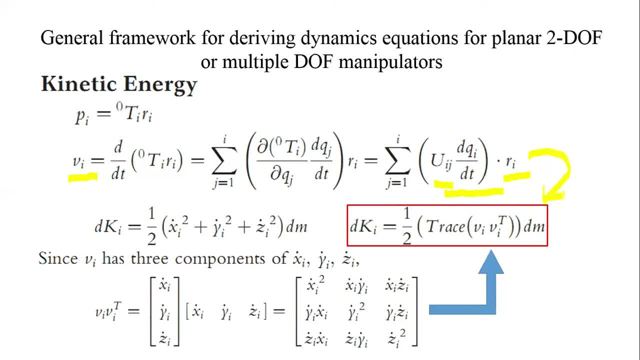 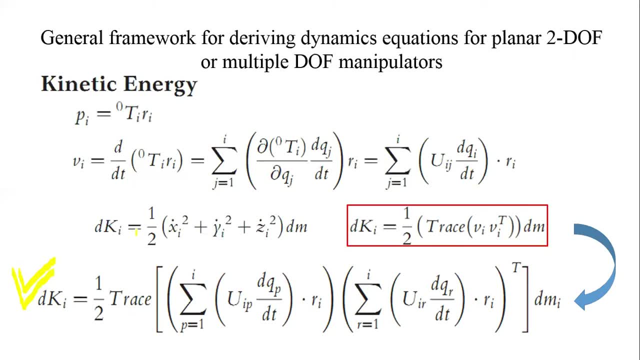 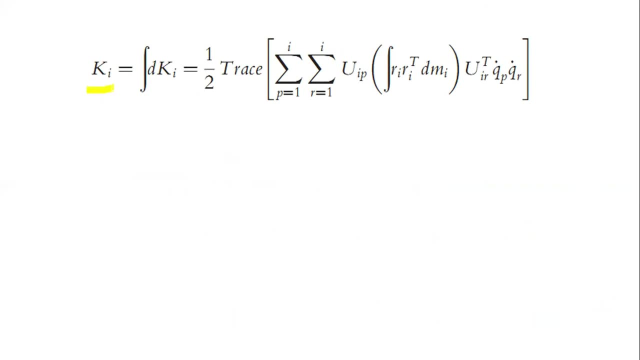 this expression into this equation, then the resulting equation will be equal to v i by d, t, u, i, j. this is the general expression of kinetic energy suitable for a manipulator having any degree of freedom. in the last slide the kinetic differential kinetic energy was obtained, so the net kinetic energy of the ith link will be integration of this differential. 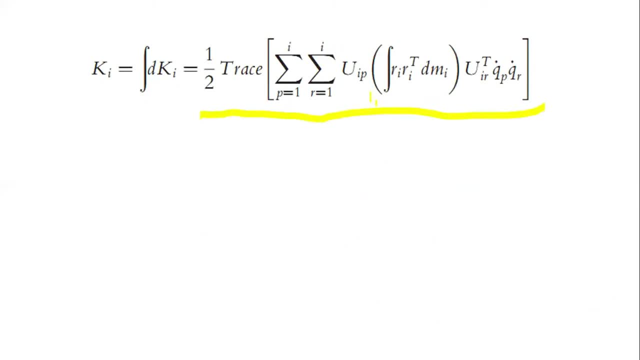 kinetic energy d, k, i, and it will be equal to this equation. this term denotes the inertia tensor and can be written. can be denoted by j, i. so the equation of kinetic energy will take this form: where j is equal to integration r i into r, i transpose into d m, i, a potential energy of the ith link can be derived in this. 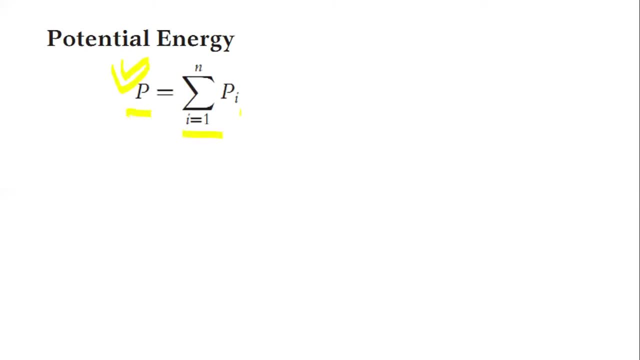 these steps, the total potential energy of the manipulator is equal to potential summation of potential energy of each link. that is equal to p. i is equal to mgh, where m denotes minus mass of the high length, then gravitational gravity vector and then position vector, the 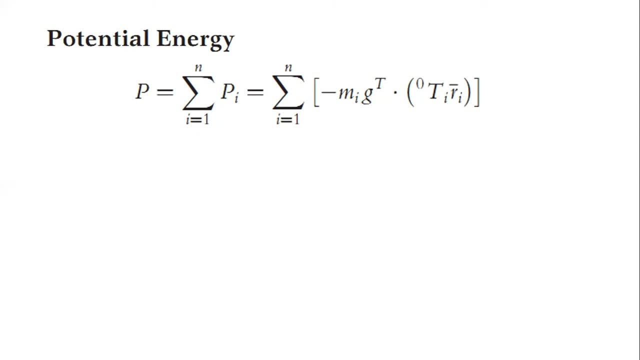 gravity vector will have three components: gx, gy and gz. g transpose is a 1 by 4 matrix and the size of this element is 4 by 1. so if we multiply mass into g, into this thing, then we will get to a still quantity. the lagrangian variable can be defined by subtracting. 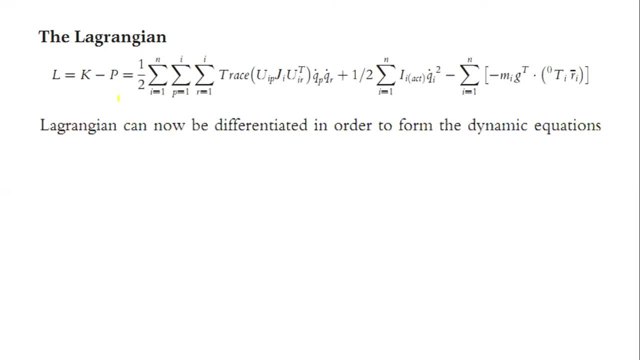 kinetic energy minus potential energy, and the expression will take this form here: lagrangian can now be differentiated in other in order to form the dynamic equation. so let's take the derivative of this equation and finally, the tor equation, or effect equation, will be like this: here the expression of dij is something like this, and we denote the inertia term because 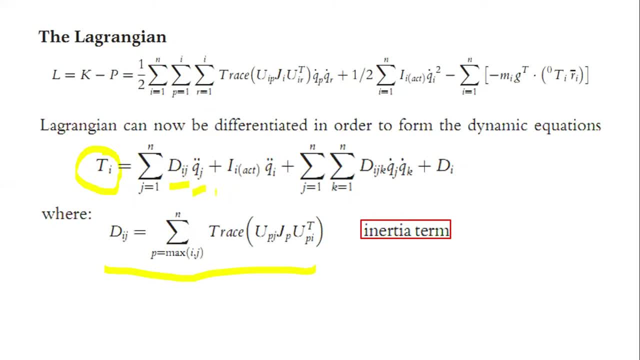 it is a multiplicable equation, now and then when we solve it. this is not just a simple applied after acceleration. so inertia into acceleration is force and again this term is inertia tensor and this dijk basically denotes a term associated with the coriolis component. dij denotes coriolis and centrifugal terms di. the expression of di is written here: 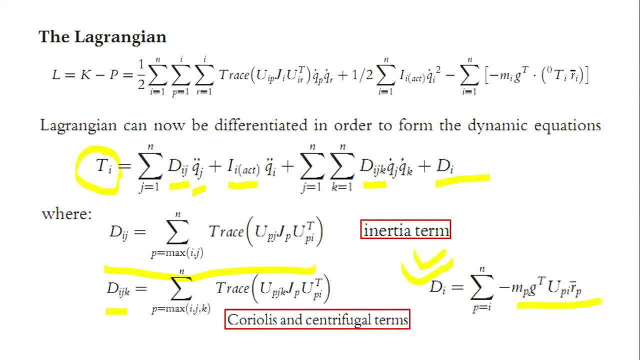 and it denotes the gravity term send. This is the general formula of manipulate dynamics: table for manipulators having degree of freedom less than two or more than two. So this is the general formula of manipulated dynamics: is table for manipulators having less than two degree of freedom or more than two degree of freedom. Let us take an example and derive. 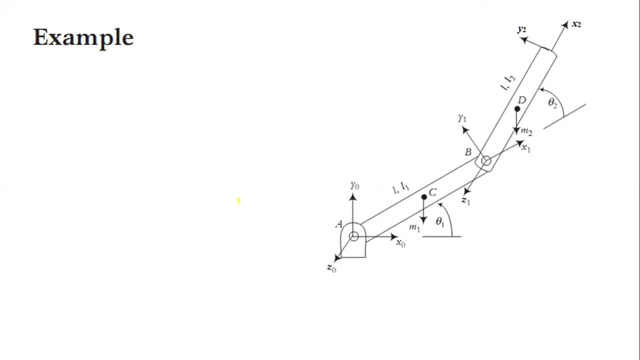 the manipulator dynamics using the general formula. So the transformation matrix of first element with respect to base will be like this and the transformation matrix of second link with respect to first sequence pair will be like this: Now if we derive the Uij, then we need to take partial derivative of the if-link with. 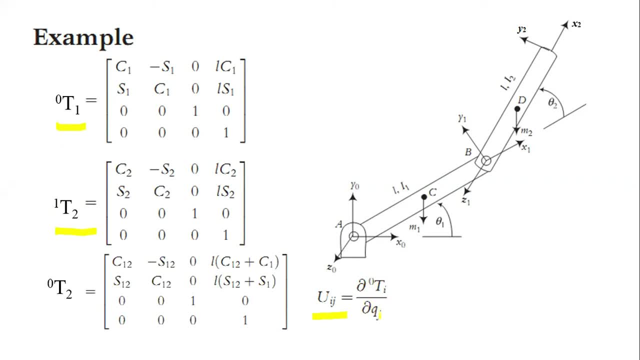 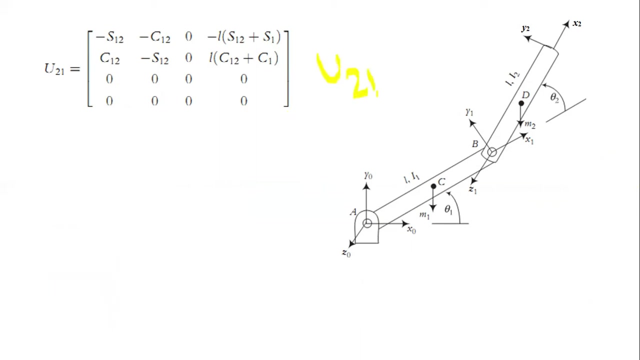 respect to zero with respect to the joint variable Qj. So U11 can be obtained by taking partial derivative. U11 will be equal to partial derivative of zero T1 with respect to del theta 1 and we will get this matrix. U21 can be calculated by the expression: U21 is equal to del zero T1. 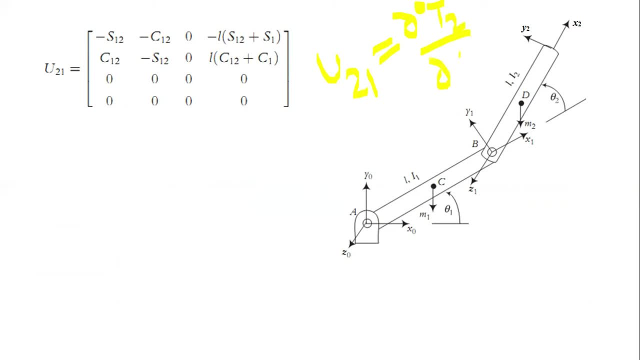 Similarly, we can derive the matrix U22 by taking partial derivative of zero T2 with respect to theta 2.. U12 will be equal to zero, and then we can find out the inertia tensor of the first link and inertia tensor of the second link. 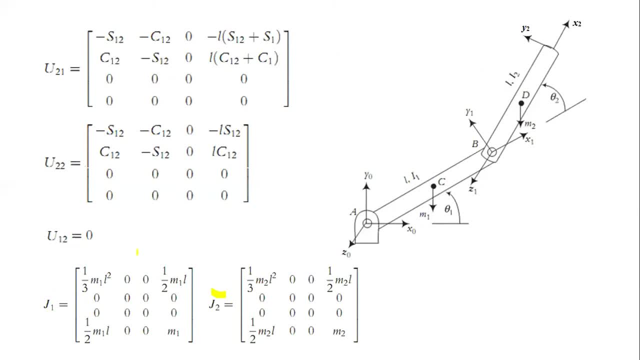 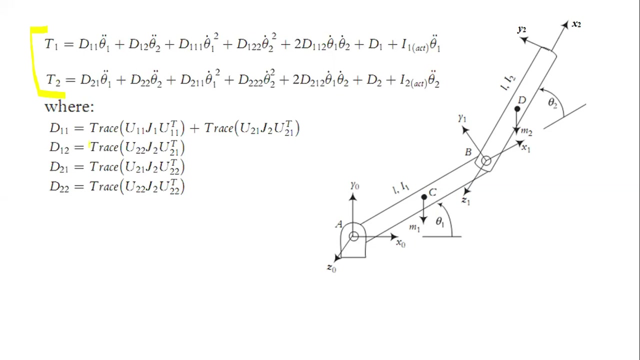 The inertia tensor can be derived, and here we can see the matrix T2.. it is not. it may be noted that the product moment of inertia is considered zero here. that means the link has been considered symmetrical. the general equation of manipulator dynamics is given here, and the term d11 can be calculated with this equation. d12, d21, d22. 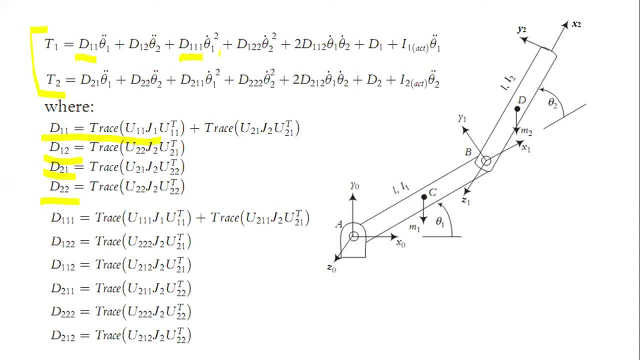 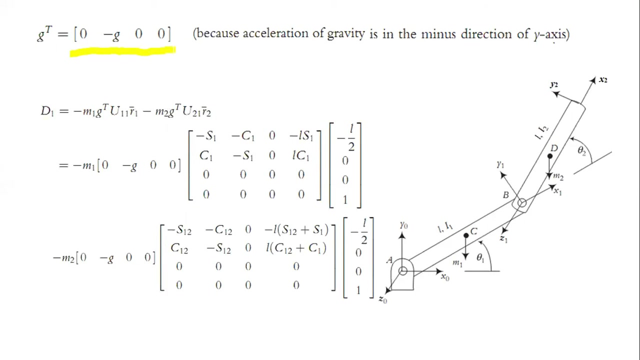 and the other variables like d11, d122, d1, 1, 2 and all the centrifugal and the coriolis coriolis terms can be calculated from these equations. the gravity term d1 and d2 can be found using these two relations. the gravity vector will be 0 minus g 0, 0 because the gravity is acting. 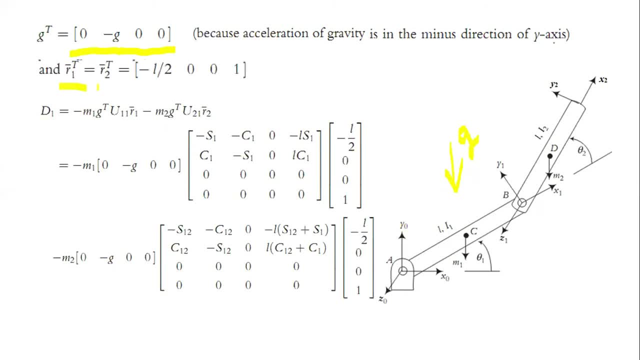 in the opposite direction of y vector. r1 and r2 denotes the location of center of mass of the first link and the second link with respect to first reference frame and second reference frame. so this is the first reference frame and the location of center of mass of the first link is at the distance minus l by 2 from. 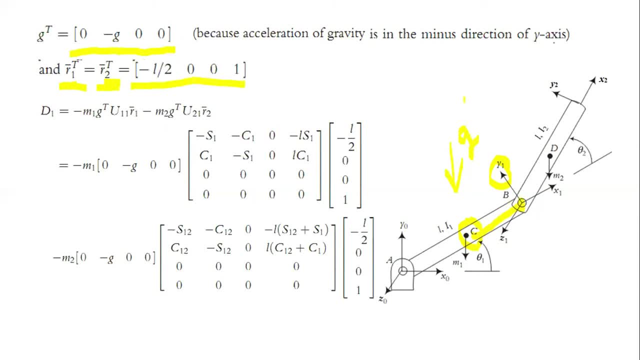 the origin. so the vector is minus l by 2 0, 0, 1. same is true for this second link. also substitute the gravity vector and these position vectors in this equation of d1 and we will find we will get the final expression of d1 and d2 just after.